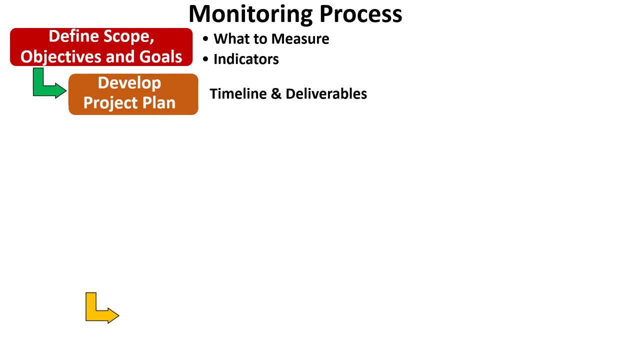 and the resource utilization with the plan. Third, it is important that there is a clear roles and responsibilities assigned to the team members. Also, communication channel needs to be established to ensure that everyone is aware of the responsibilities and there is a continuous flow of information regarding the project implementation. 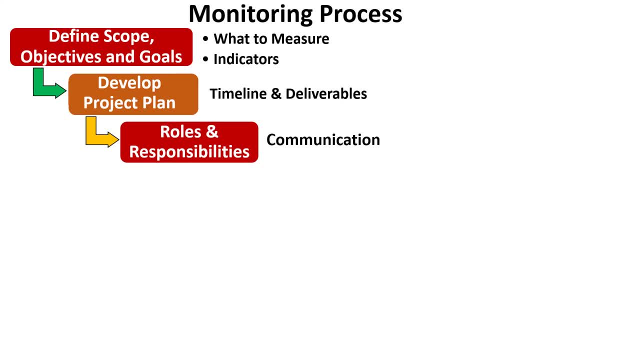 Regarding the project, its issues and progress. At number four, we need to develop the monitoring system which will enable us to track the progress against the project plan. Monitoring system can take a form of regular status report, checkpoint reports, progress reports or reporting against some standard formats. 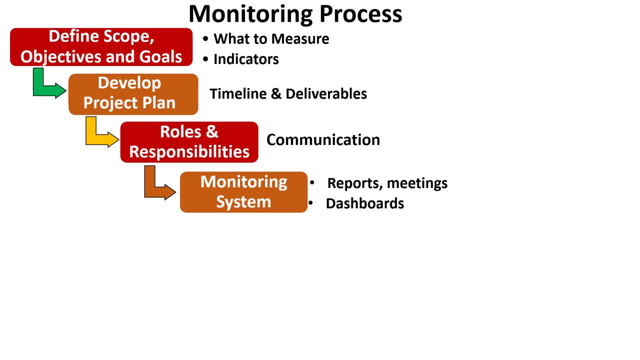 including dashboard reports. After having the monitoring system in place, we can start collecting the data on the project, performance and progress, including financial data and issues or risk that may arise. Having collected the data on the project, it needs to be analyzed so as to see how. 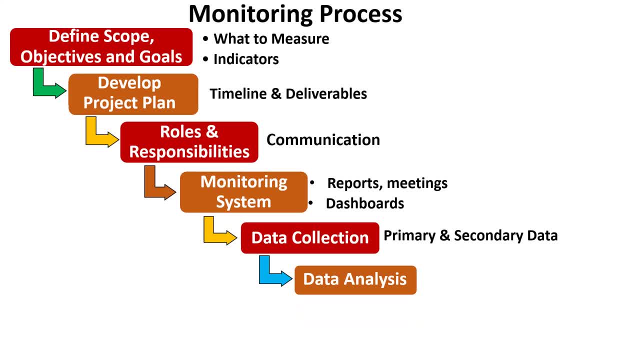 the project is progressing. The progress data needs to be compared with the milestone or the plan to understand the project progress against the objectives. The data can be used to identify trends and patterns, understand the risk and bottlenecks that the project may face and to 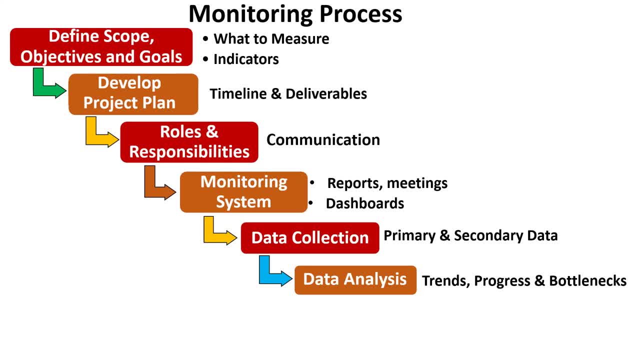 address the needs of the project. The data can be used to track the progress in the project. The second part of the project is the improvement. Ultimately, we need to communicate the progress of the project to stakeholders, including the team members. We also have to take corrective actions. 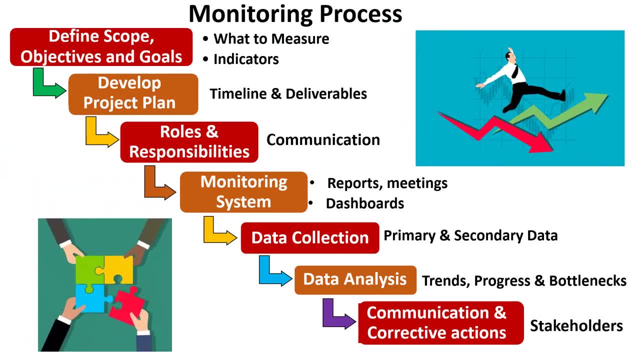 if the project is not progressing well, Corrective actions may include reallocation of resources, revising the project plan, adjusting the timelines and correcting other bottlenecks. This should help project get on track. in conclusion, monitoring a project needs to be systematic, where actual progress is tracked against the project plan data.